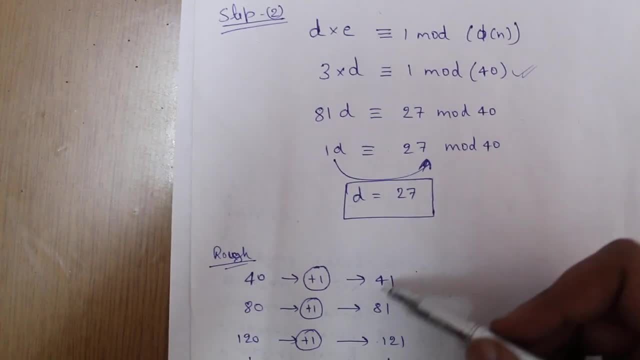 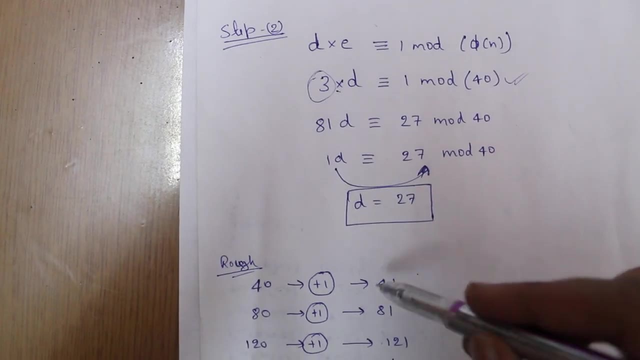 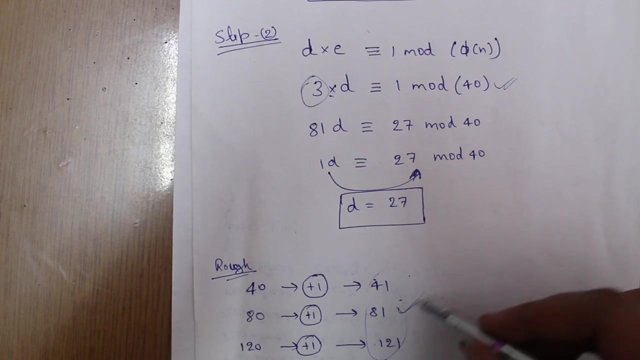 1 is 121.. Now we have to compare these values with this value, E value. If E completely divides this value, any of the given value, then we will take this value. So here, 81 is completely divisible by 3.. So if we will put this here: 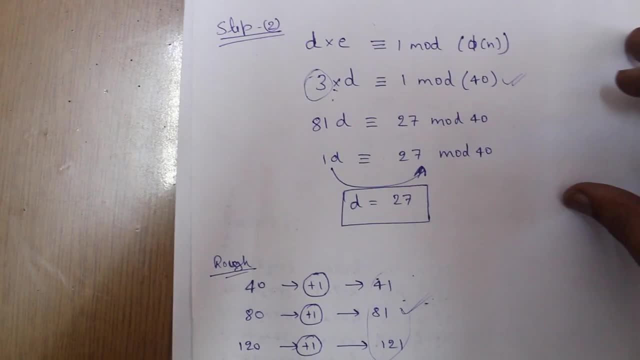 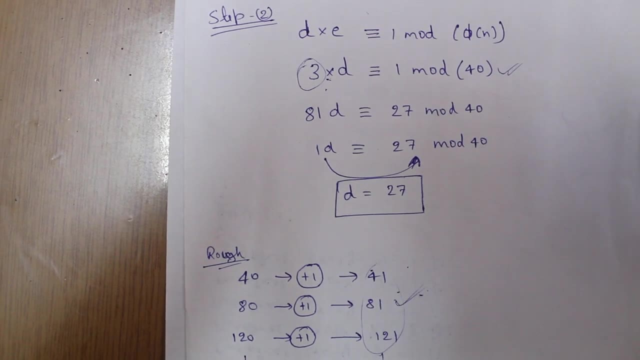 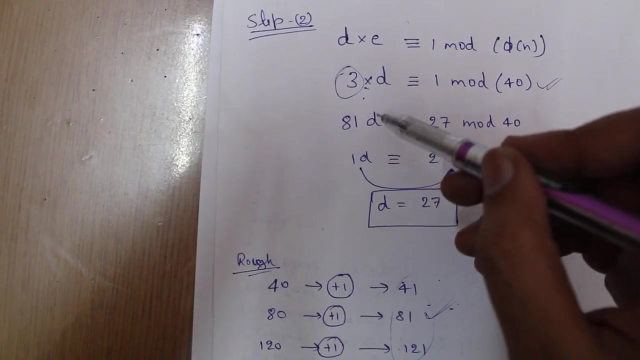 We will get 1 as the modulus value, So we have to make this equation equivalent to 81. So what will the number which will multiply so that this equation will be equivalent to 81. So 27 is the number. if we will multiply here, then it will be 81. So we will multiply. 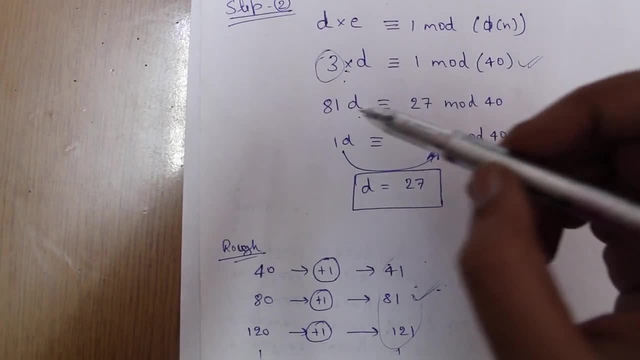 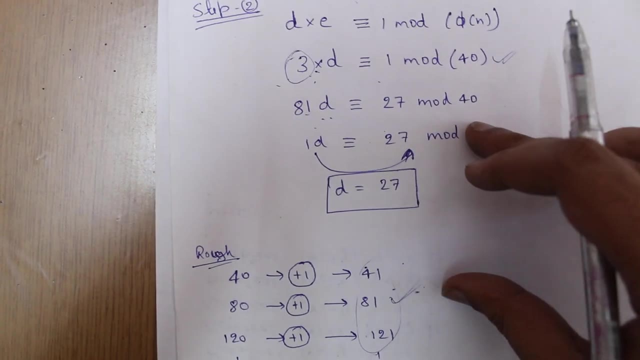 this equation with 81. Sorry, 27.. So it will be 81.. 27 into 3 will be 81. And here it will be 27.. And mod 40 will remain the same. Now, if we will take 40 into 2,, the modulus of 81, we 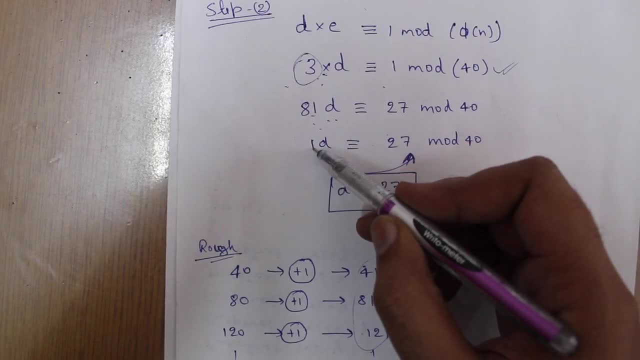 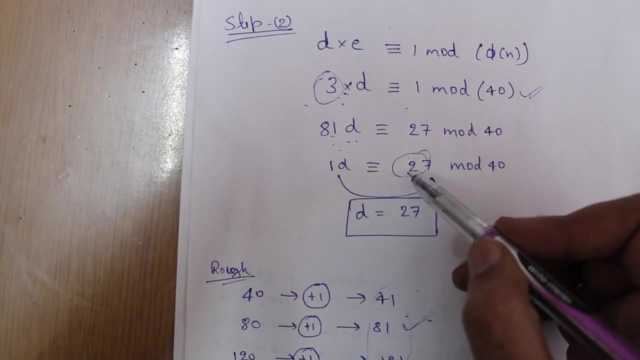 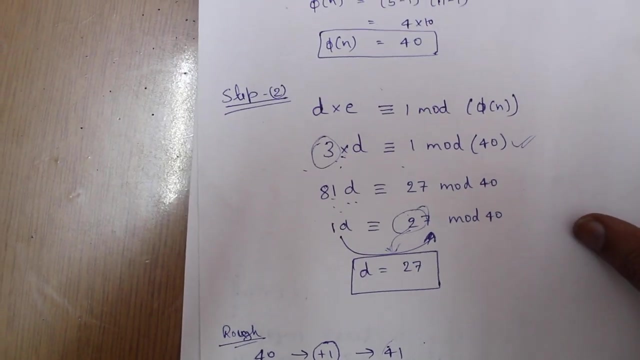 will get 1 as a remainder When the product value with the d will be 1, then this value will be equal to d. So this is a very simple concept And it is just a two-step process. Now we will again take another value. So this is a very simple concept And it is just a 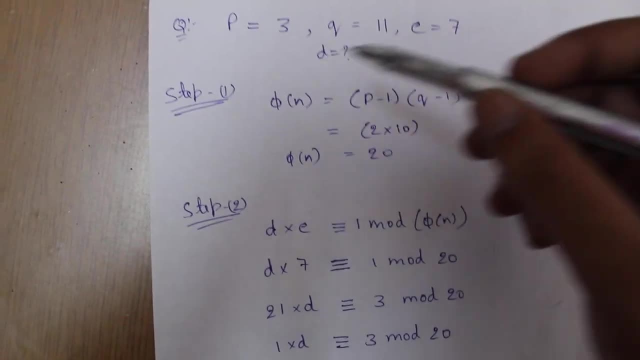 two-step process. So this is a very simple concept And it is just a two-step process. And it is just a two-step process. Now, if we come back to another example, Lets p equal to 3.. q equal to 11. And e equal to 7. So here we also have to calculate the 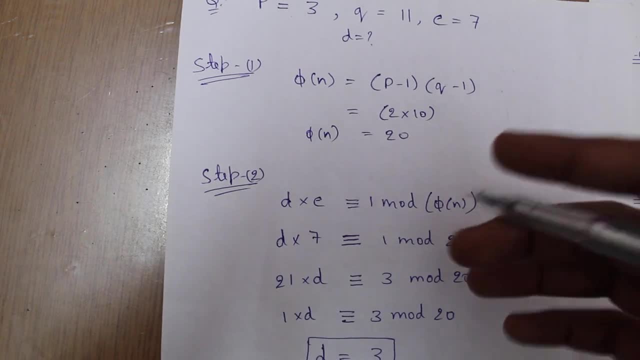 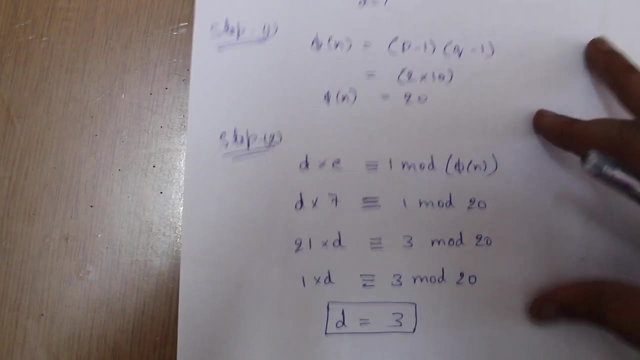 d with the d. So the first step is: can we have to calculate the phi in value? It will be 3-1, which is 2, with 11-1, which is 10.. So it will be 20.. Now the step 2.. We will put the values which are given And then we will get the d into. 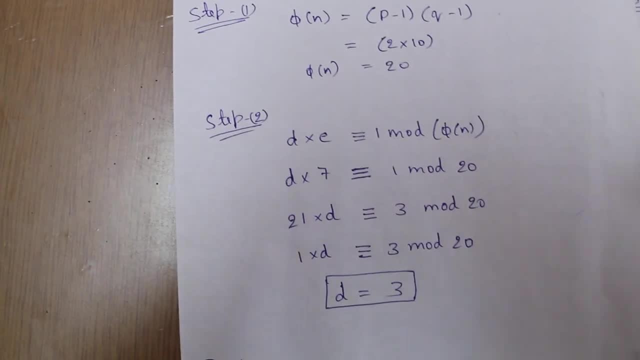 7, which is one mod 20.. We have come to the final product: gourre. let's say 1 by 21.. How much you should multiply 3 by 21? or Sp统, thechs, thechs, thechs, thechs. 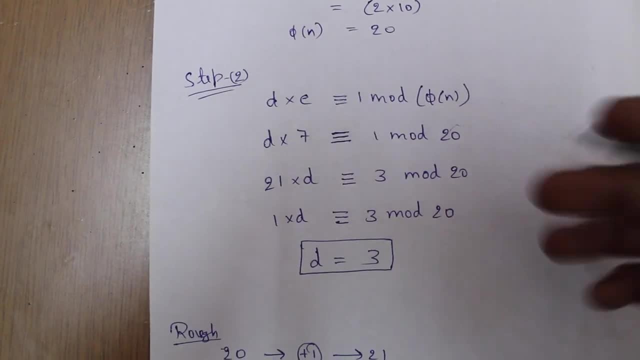 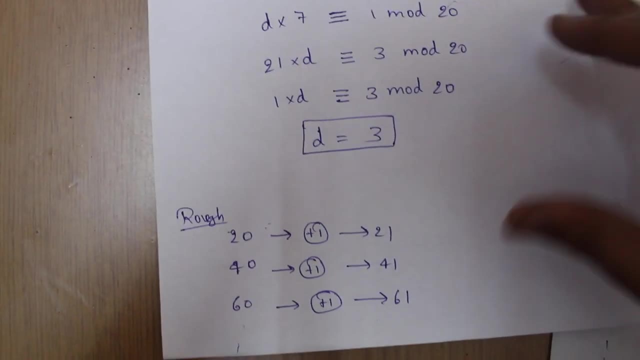 q,3q and h. you should multiply. told you earlier that we have to write the table of the 5 ins side by side, so it will be 20, 40, 60 and dot, dot dot. continue the same process and also we will add 1 in each number.